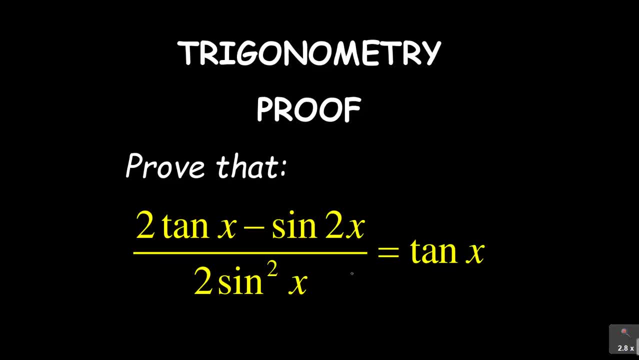 x is equal to 10x. So this is the question that I took from one of the previous papers, and you are required to prove that Now, before we begin our lesson. I will encourage you, guys, if you want to get some more of these. 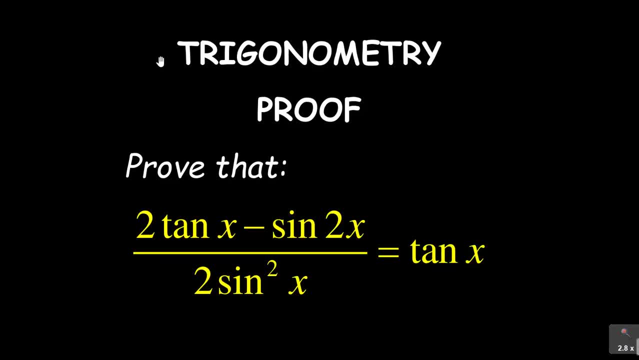 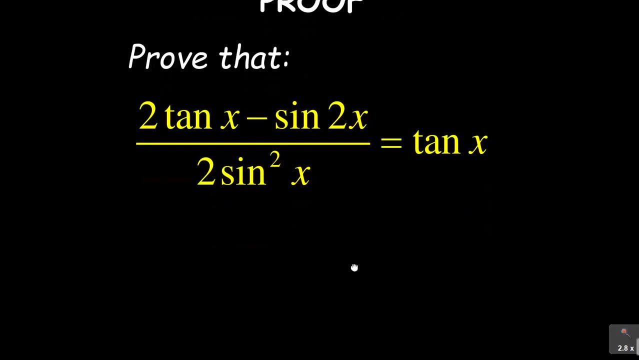 revision sessions. please subscribe to our channel And the most important thing to do there is to turn that notification bell on so that you're notified. every time there's a new video, YouTube will notify you. Now let us dive into this proof. What I'm given here is: whenever you're proving, remember you have to choose the site which. 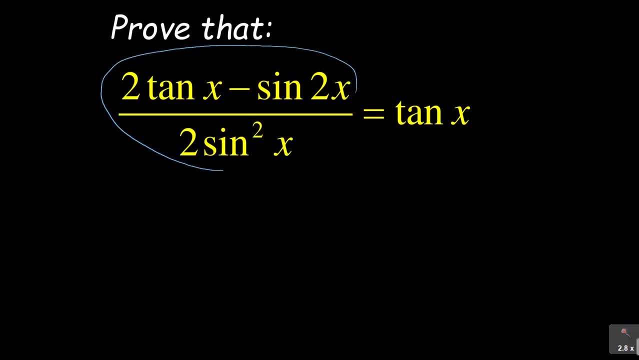 you want to study And from what I have, this has got more for me to work on. So I'm going to choose my left hand side. So that's what I have, left hand side, And I'm going to write the left hand side, which is 210 x minus sin, two x all over two. 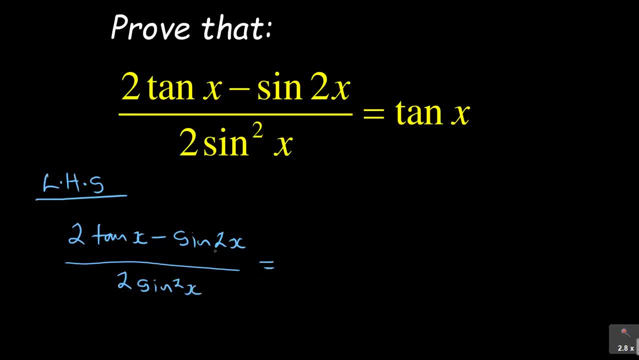 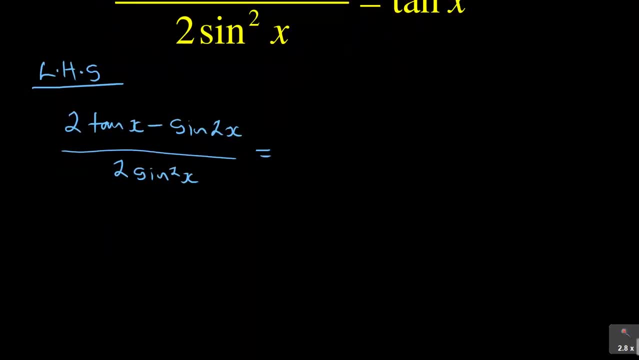 sin squared x, this is equal to, so I'm going to work it from there. remember, the aim is to prove that that is 10x. So this is equal to. now I need to know my basic arm. I'm just going to have it at the bottom here while I'm working on it. 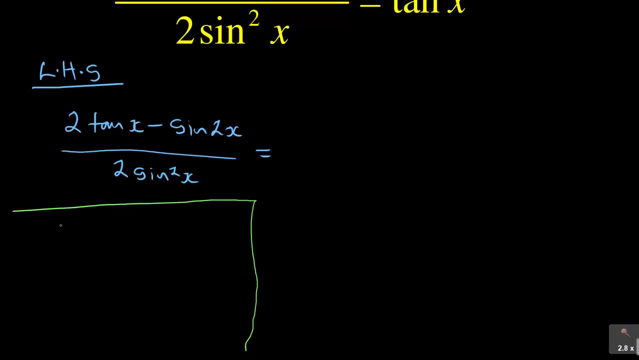 So I need to know my basic trick identities. For example, you need to know that 10x is equal to 10x, Sin x over cos x. So these are the most basic identities that you need to know, which you will not be provided. 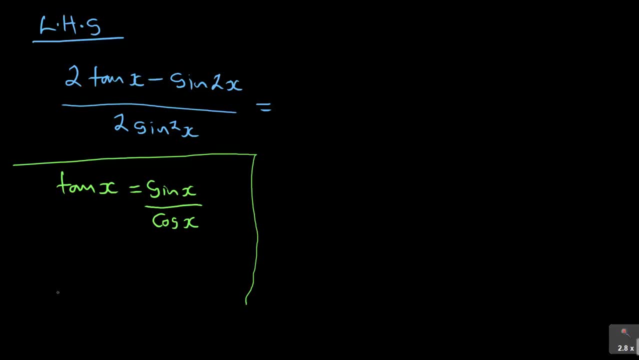 in your exam. And the other one, which is also important, is sin squared x plus cos squared x is equal to one. These are very, very important for you to know. So now let us continue, then, With our question. so 210 x now for 10, we're going to say two, and then we have sin x over. 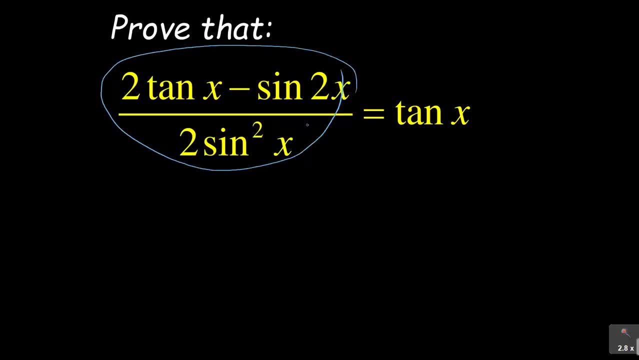 And from what I have, this has got more for me to work on. So I'm going to choose my left hand side. So that's what I have, left hand side, And I'm going to write the left hand side, which is 210x minus sin 2x, all over 2 sin squared x. 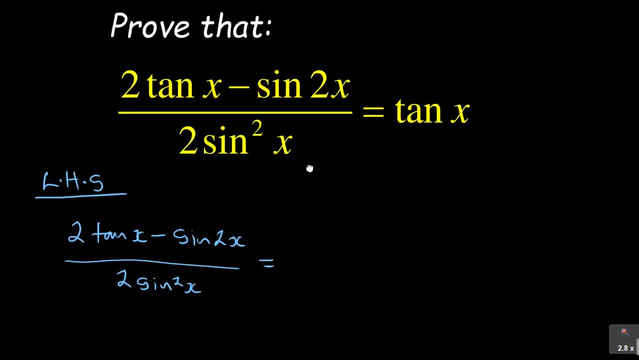 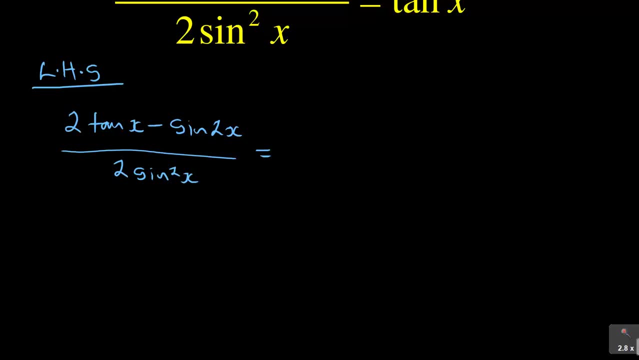 This is equal to, so I'm going to work it from there. Remember, the aim is to prove that that is 10x, So this is equal to. now I need to know my basic. I'm just going to have it at the bottom here while I'm working on it. 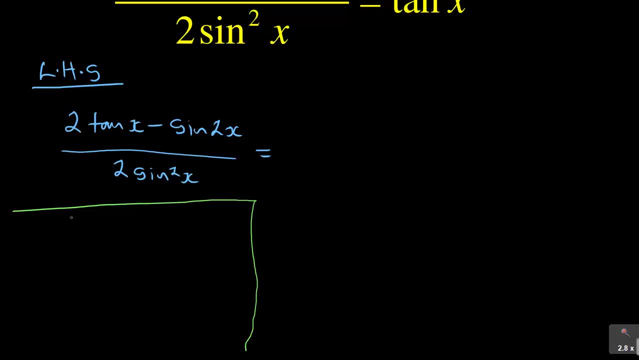 So I need to know my basic trig identities. For example, you need to know that 10x is equal to sin x over cos x. So these are the most basic identities that you need to know, which you will not be provided in your exam. 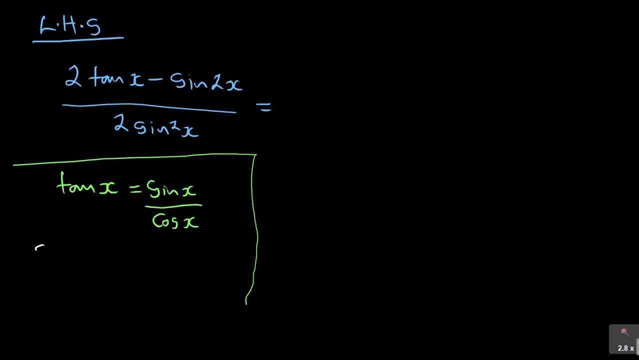 And the other one, which is also important, is sin squared x plus cos squared x is equal to 1.. These are very, very important for you to know. So now let us continue, then, with our question. So 210x, Now for 10,. 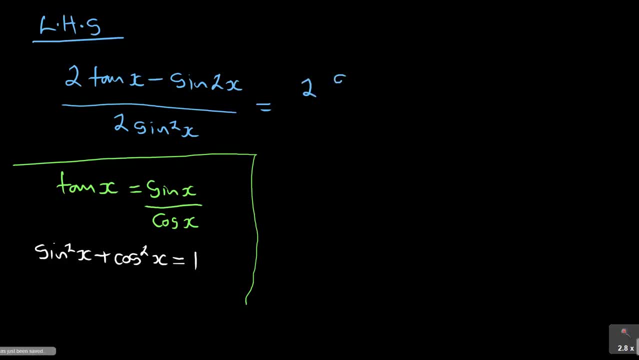 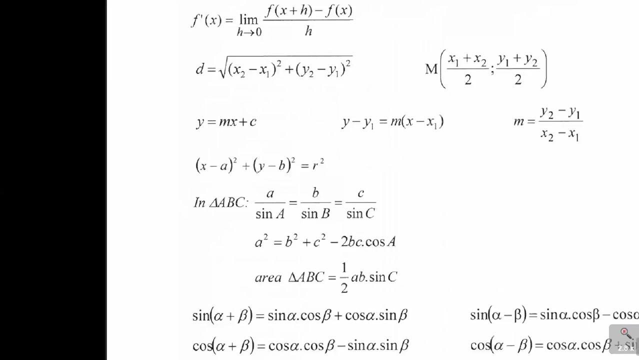 we're going to say 2, and then we have sin x over cos x instead of 10.. And then we have minus. now sin 2x. We can further simplify sin 2x if I go to my formulas And if I just zoom in and you can see that I have the identity for sin 2x. 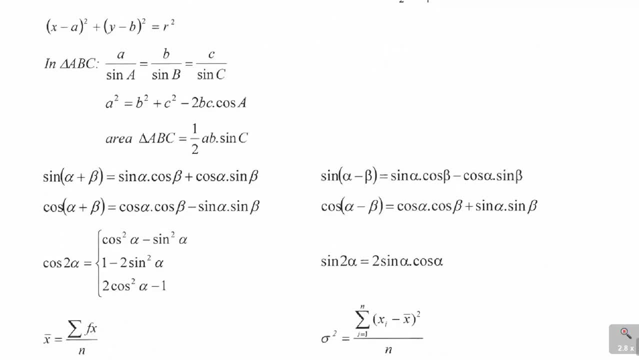 In this case it's 2 alpha. If you look at it, there is the one for 2 alpha which says sin 2 alpha is 2, sin alpha cos alpha. So that's what I'm going to use. So this is minus. 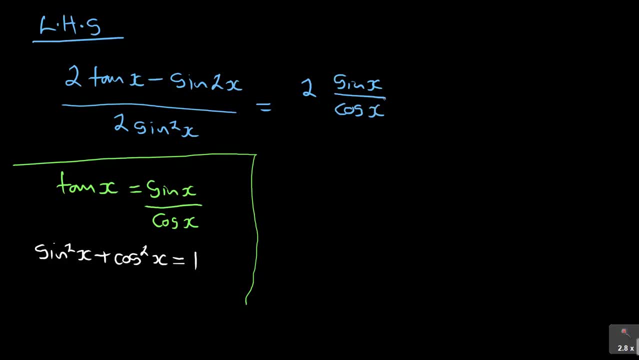 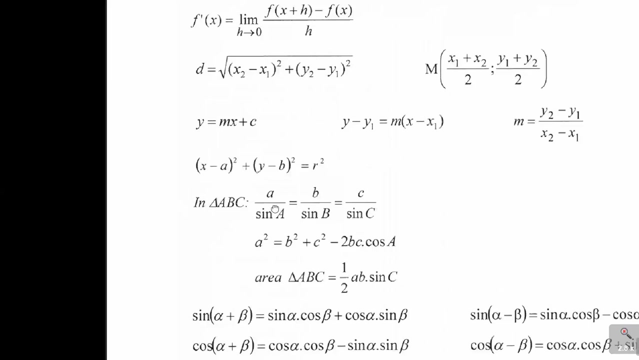 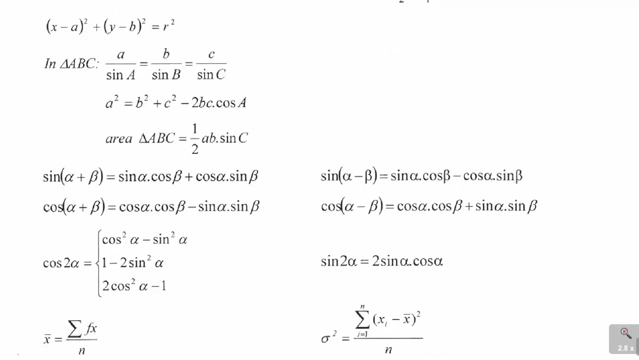 cos x instead of 10.. And then we have minus, now sin two x. we can further simplify sin two x if I go to my formulas And if I just zoom in and you can see that I have the identity. The identity for sin two in this case is two alpha. if you look at it, there is the 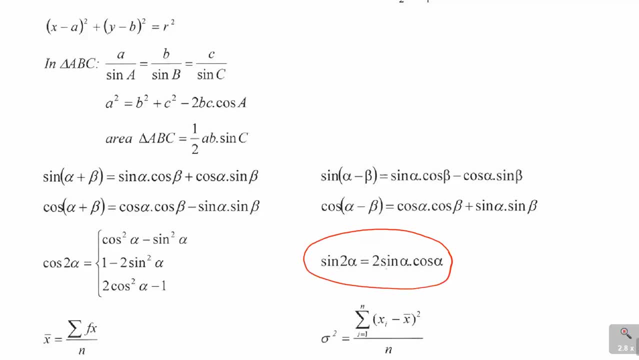 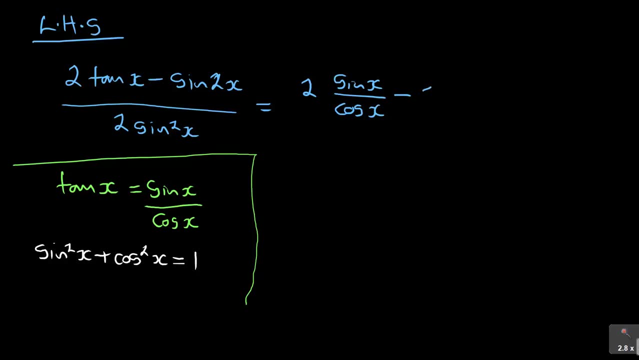 one for two alpha, which says sin two alpha is two. sin alpha, cos alpha. So that's what I'm going to use. So this is minus. And then I'm going to use two sin x, cos x, And it says I must divide everything here. 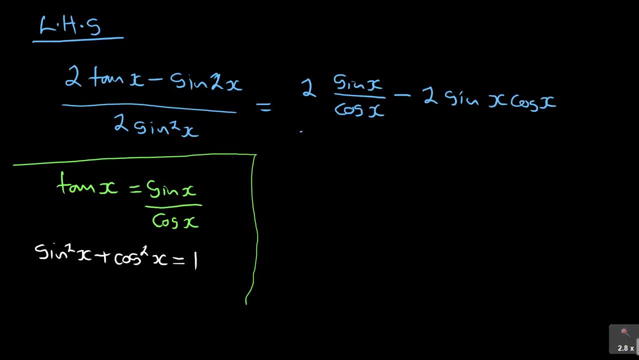 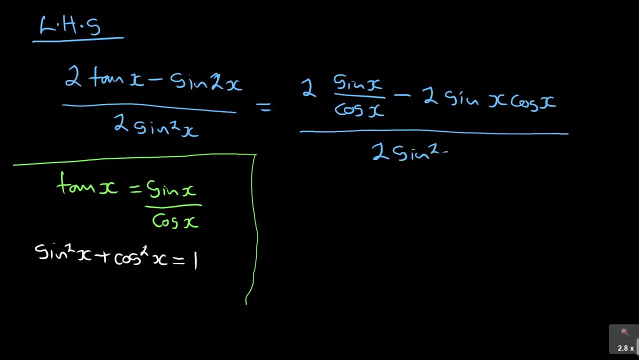 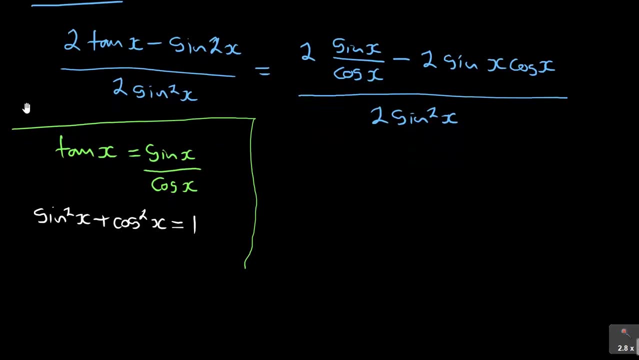 And then I'm going to use two sin x, cos x. So now, when I choose two here at this point, the next step will be to divide everything here by two sine squared x. Now, what I want to emphasise also here is, when you're given a fraction, just want to. 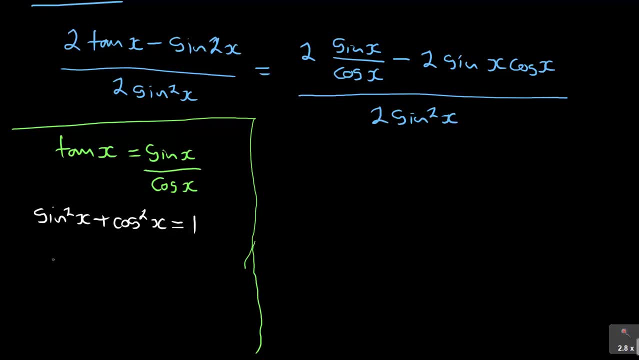 show you something here. when I'm given a fraction, for example, let's say I'm given sine x plus cos x and then it's over 10 x, And then I'm going to use these positive fractions. So here I'm just going to use them in the model which is equal to two times sin x plus. 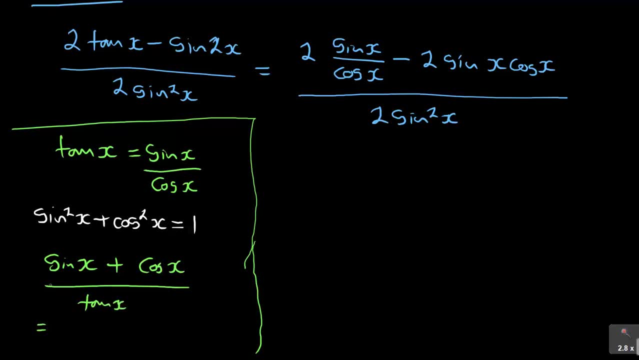 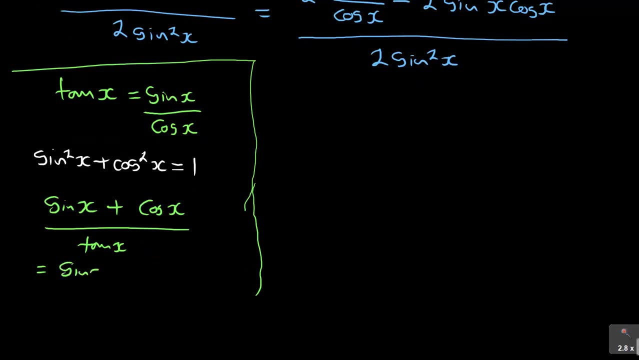 cos x. And then let's go on What it means. I can simplify this and say this is same as saying the 10 is affecting the sine, so it will be sine x over 10x plus. again the 10 is affecting the cos because 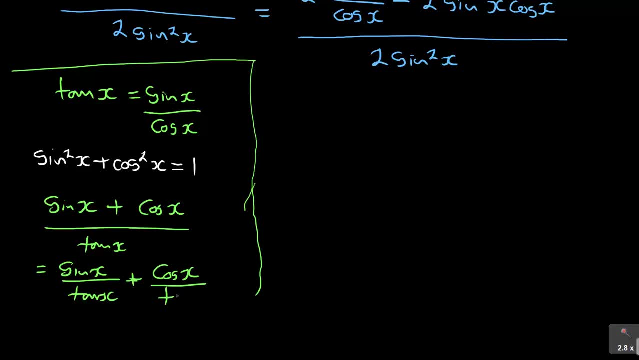 of the plus sign, which is cos x over 10x. So this means that is what it means here whenever we are working on the fraction. So, using the same concept, I'm going to then distribute the denominator, which is the 2. 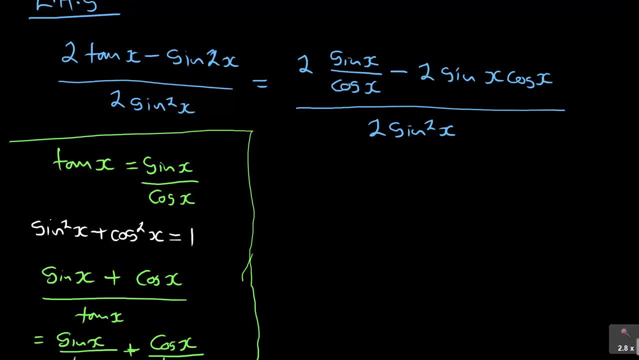 sine squared over the two numerators, which will be equal to 2 sine x over cos x. Now I'm going to say all over 2 sine squared x, as we said, and then minus, actually the minus It can be here, minus which is 2 sine x and cos x, all over 2 sine squared x. 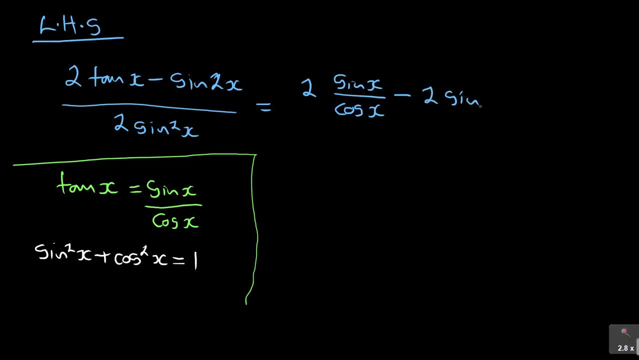 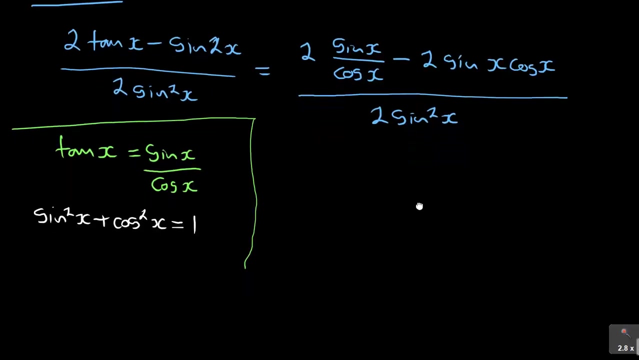 And then I'm going to use 2 sin x, cos x, And it says I must divide everything here by 2 sin squared x. Now, what I want to emphasize also here is when you are given a fraction. just want to show you something here. 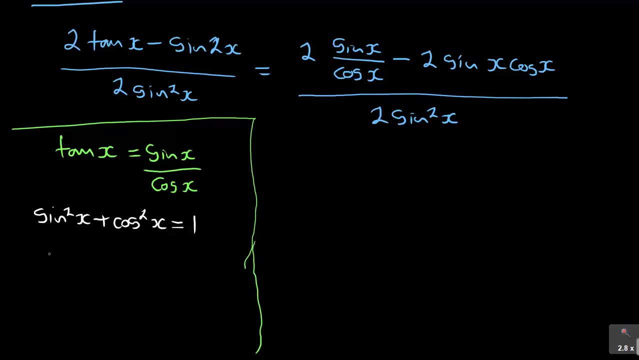 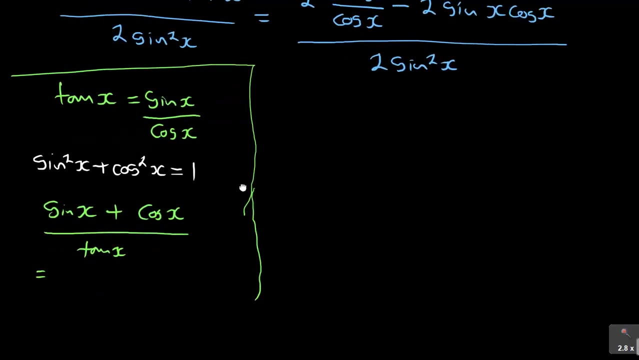 When I'm given a fraction, for example. let's say I'm given sin x plus cos x And then it's over 10x What it means. I can simplify this and say this is same as saying the 10 is affecting the sin. 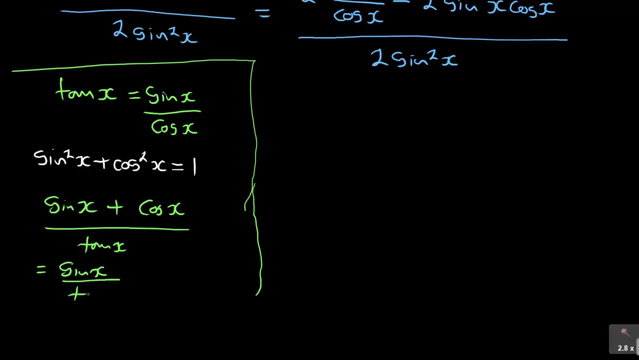 so it will be sin x over 10x Plus. again the 10 is affecting the cos because of the plus sign, which is cos x over 10x. So this means that is what it means here whenever we are working on the fraction. 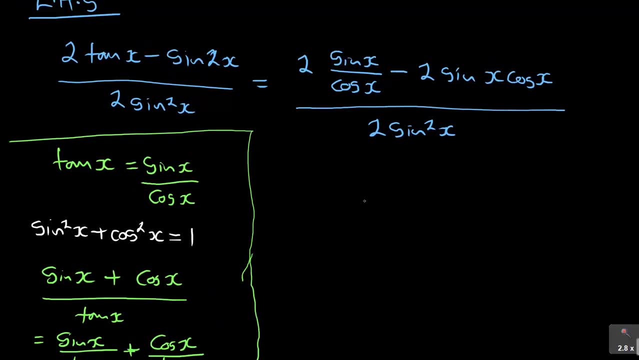 So, using the same concept, I'm going to then distribute the denominator, which is the 2 sin squared over the two numerators, which will be equal to 2 sin x over cos x. Now I'm going to say all over 2 sin squared x. 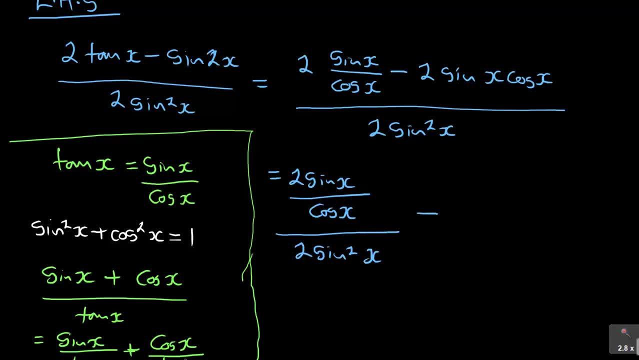 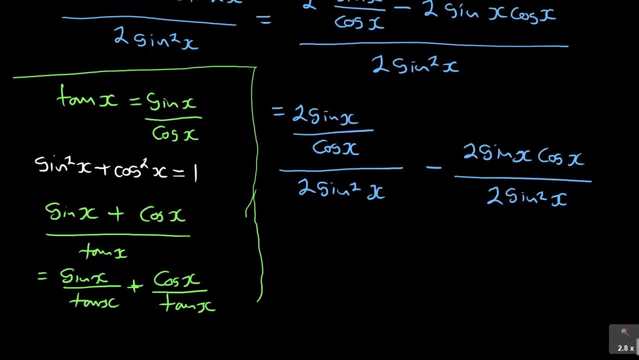 as we said, and then minus. actually the minus can be here, minus, which is 2 sin x and cos x, all over 2 sin squared x. So you see how I've managed to distribute that denominator there into both. Now what I'm going to use. 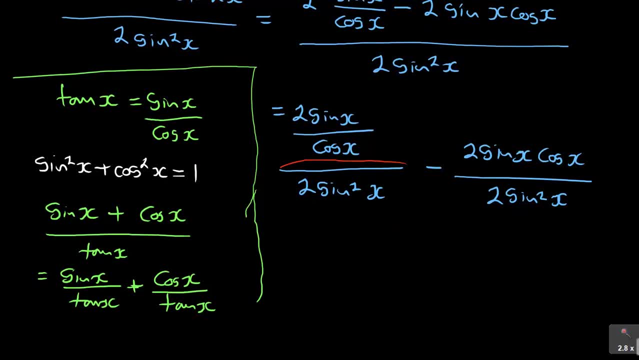 I'm going to convert this particular division into a division sign, so that I mean a division sign such that I have equal to 2 sin x over cos x, And then I'm going to turn it to divide it, as I was saying like that. 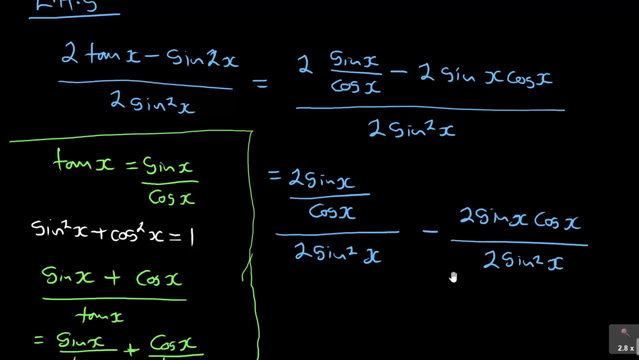 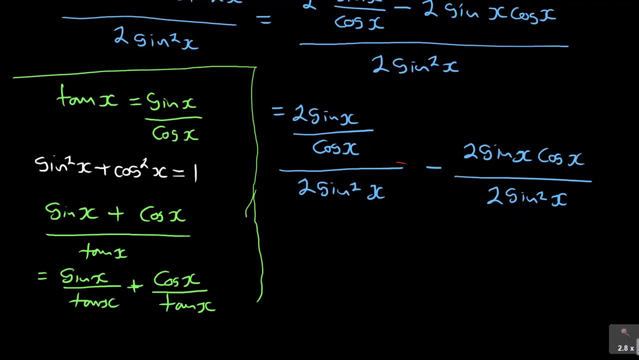 So you see how I've managed to distribute that denominator there into both. Now what I'm going to use, I'm going to convert this particular division into a division sign, so that I mean a division sign such that I have equal to 2 sine x over cos x. and then I'm going to 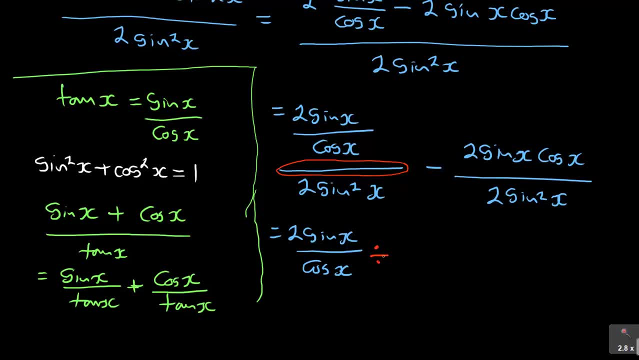 turn it to divided, as I was saying like that, into that division sign: divided by 2 cos squared x, and then I mean 2 sine squared. it's not cos squared actually, it's 2 sine squared x. 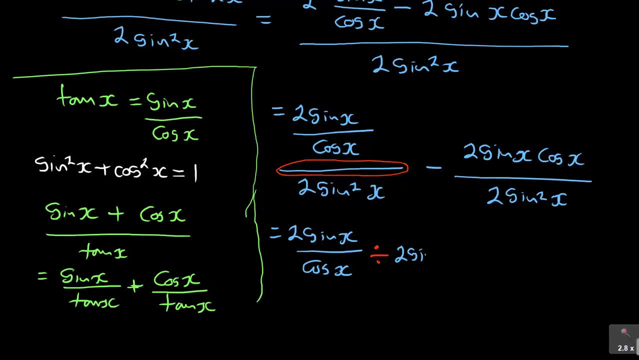 That's what I'm dividing with, which is 2 sine squared, x and minus. I just I can actually simplify what I have here without much, so the 2 will cancel there. Now I've got sine x on top and then I've got sine squared, which means there are two. 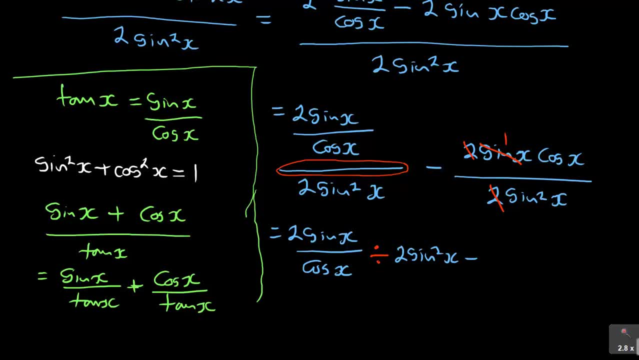 of them at the bottom. So 1, I will cancel there, and from 2, I will be left with 1.. So what I have then is minus cos x over sine x. That's what I'm having on the other side. 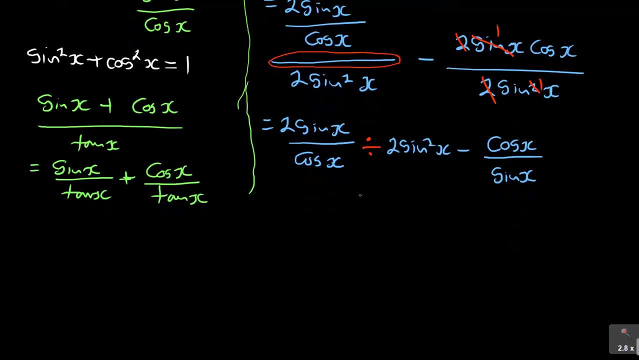 And then this can continue to be equal to 2 sine x over cos x- Remember, that was our 10 in that case. And then from divided to multiplication- remember, when I'm dividing, I will then multiply. Now it was 2 sine. 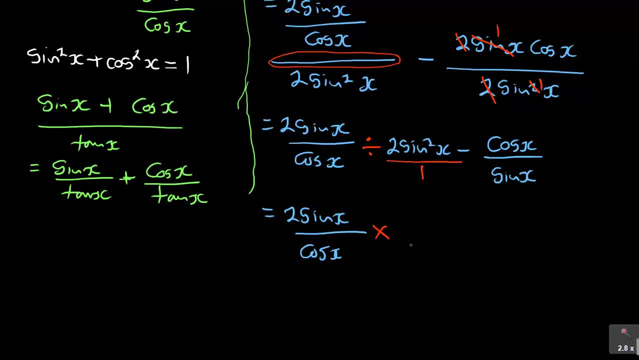 x squared over 1.. So when I divide it will be 1 over and then you will have 2 sine squared x. Then it's minus cos x over sine x, Remember that- And then this is equal to now, because I was now dividing. I'm able now to cancel the. 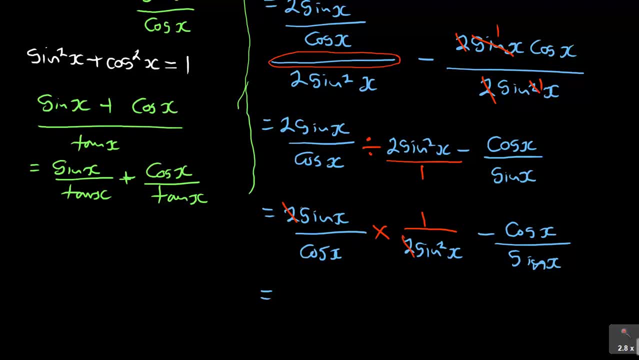 2. Again, we'll cancel the 2.. Now I've got sine x canceling the squared so that there is 1 remaining. So at the bottom now I will have on top it's 1 times 1, which is 1 over cos x, which 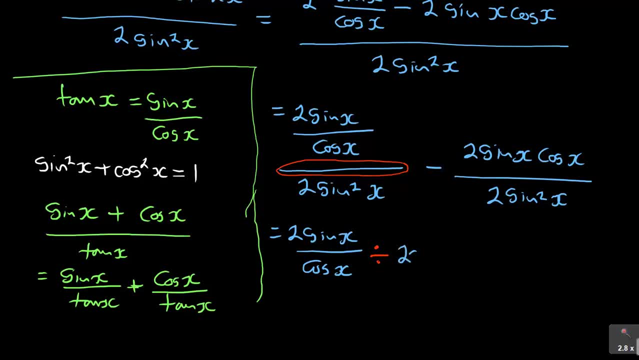 into that division sign divided by 2 cos squared x, And then I mean 2 sin squared. it's not cos squared, actually, it's 2 sin squared x. That's what I'm dividing with, which is 2 sin squared x and minus. 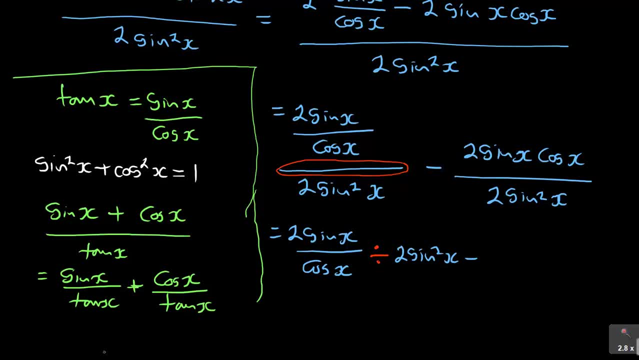 I just I can actually simplify what I have here without much. So the 2 will cancel there. Now I've got sin x on top and then I've got sin squared, which means there are two of them at the bottom. So 1, I will cancel there. 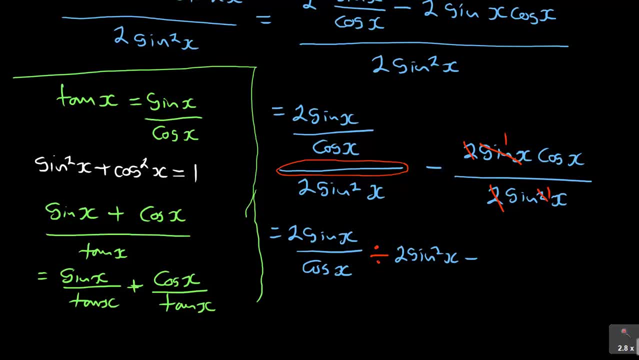 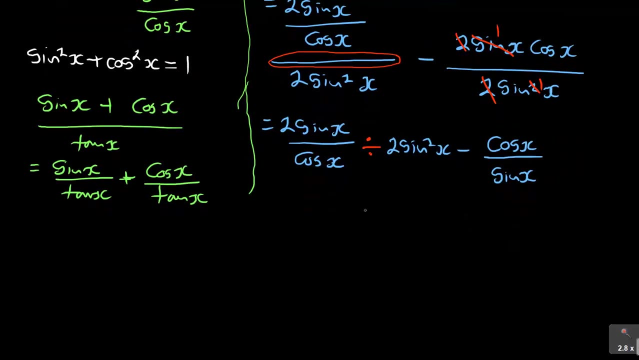 And from 2, I will be left with 1.. So what I have then is minus cos x over sin x. That's what I'm having on the other side, And then this can continue to be equal to 2 sin x over cos x. 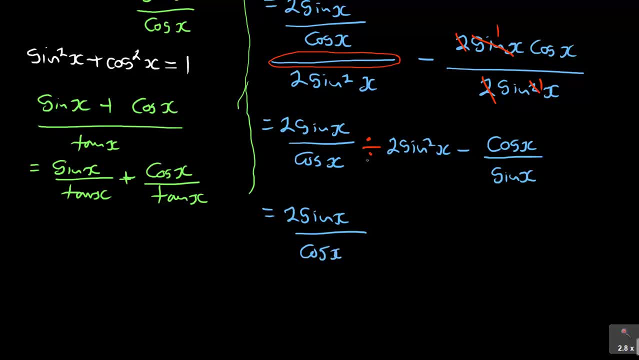 Remember that was our 10 in that case. And then from divided to multiplication- remember, I'm dividing, I will then multiply. Now it was 2 sin x squared over 1.. So when I divide it will be 1 over. 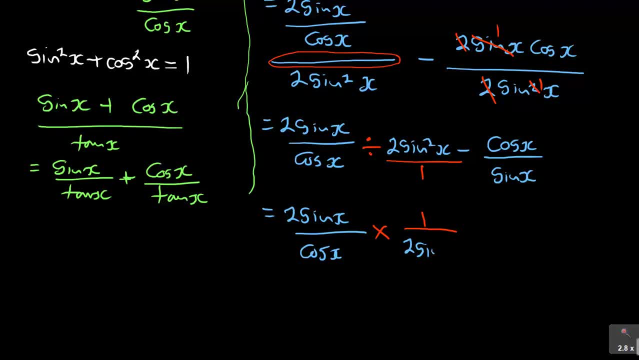 and then you will have 2 sin squared x. Then it's minus cos x over sin x, Remember that. And then this is equal to now, because I was now dividing. I'm able now to cancel the 2.. Again, we'll cancel the 2.. 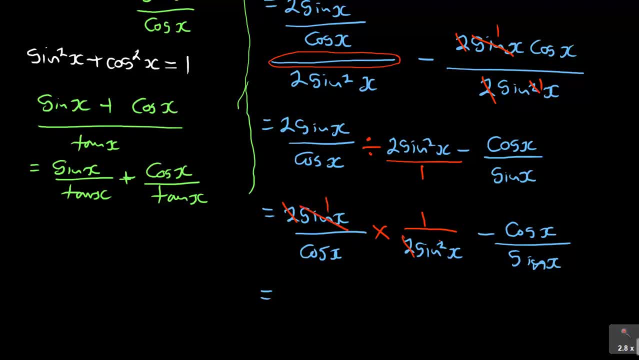 Now I've got sin x canceling the squared so that there is 1 remaining. So at the bottom now I will have: on top it's 1 times 1, which is 1 over cos x, which is that: 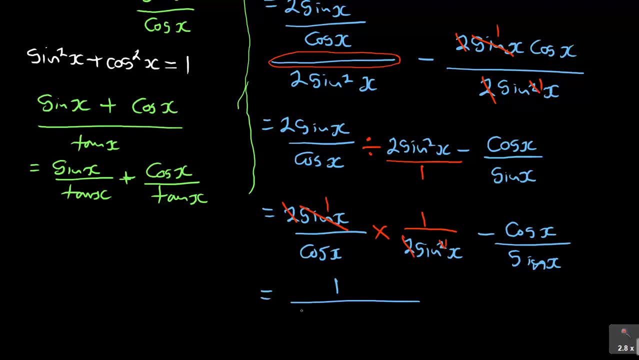 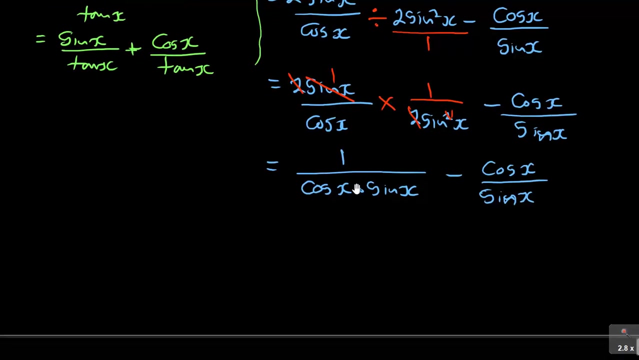 and sin x, which is that. So that is what is remaining. So which is cos x times sin x Minus cos x over sin x? So that is what we are left with at the moment. So, if we continue to simplify, 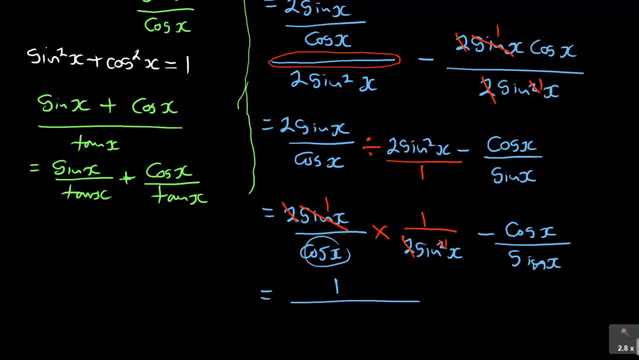 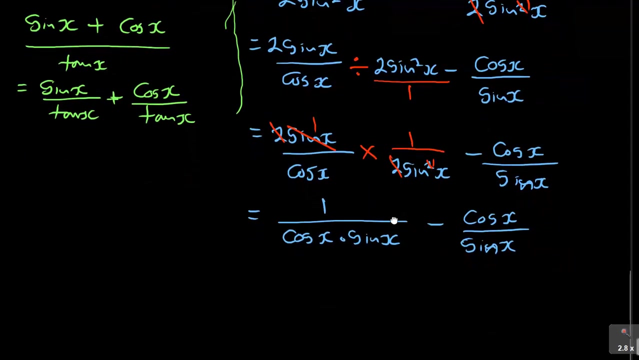 is that, and sine x, which is that. So that is what is remaining. So which is cos x times sine x, minus cos x over sine x. So that is what we are left with at the moment. So, if we continue to simplify, this part is again the common denominator between the two. 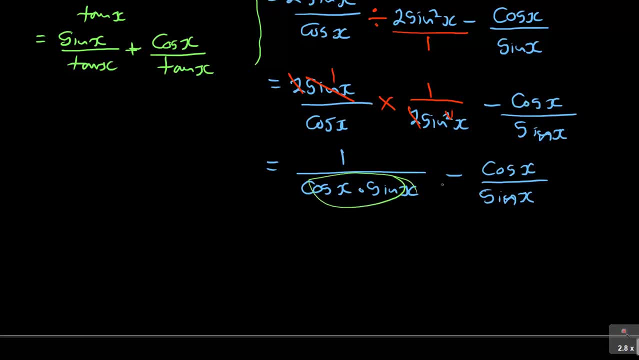 So if I focus on cos x, sine x and sine x, the common denominator in this is cos x. I'm just going to do the common denominator, which is cos x times sine x. That's the common denominator And this is the common denominator. 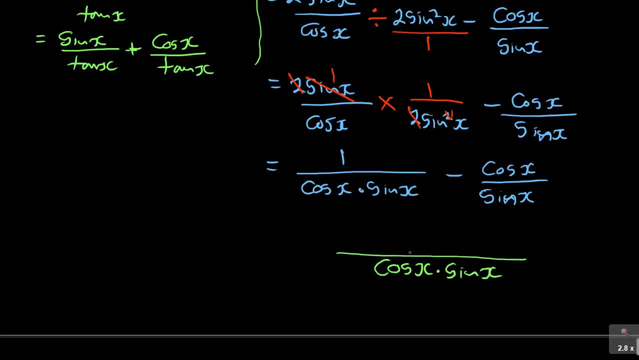 x. so that is the common denominator and you need to know fractions. so cos x sine x into cos x. sine x is equal to 1, 1 times 1. minus sine x into cos x. sine x will be the sine x will cancel the sine x, so that there is cos x remaining, and then times the numerator, which is cos x. so that is what is. 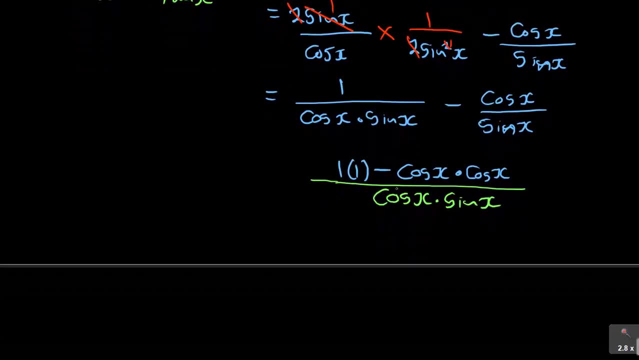 still remaining on top. so when i simplify that 1 times 1 is equal to 1 minus cos squared x all over, and then i've got cos x, dot um sine x. and then this continues to say: now i've got 1 minus cos squared x and, as i said previously, you need to know such identities now. look at this: 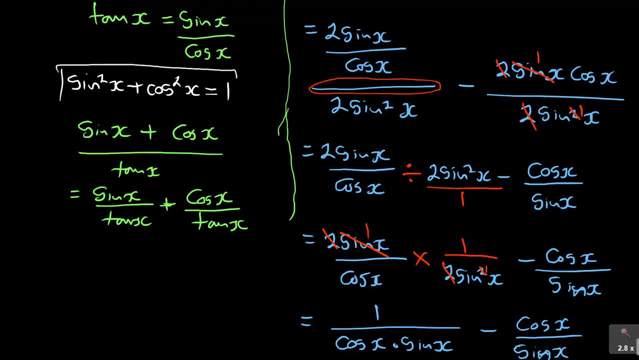 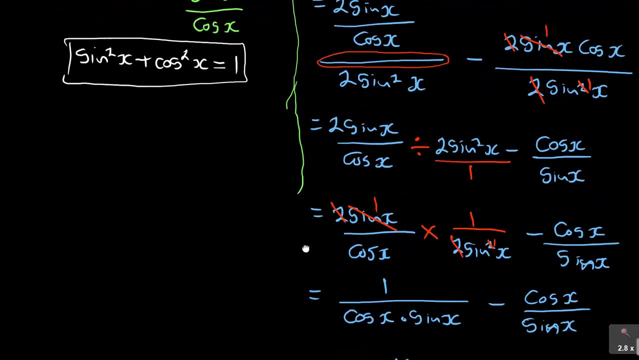 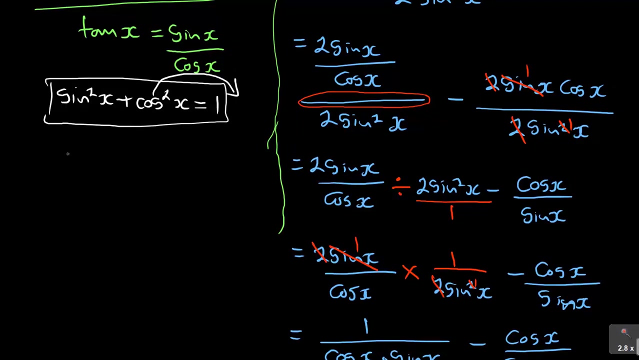 identity, which is sine squared x plus cos squared x, and if i can write it in by taking, for example, the sine squared. let me just check here by taking: yes, if i can take the cos squared instead to the other side of the equal sign, i will have um sine squared x is equal to 1. 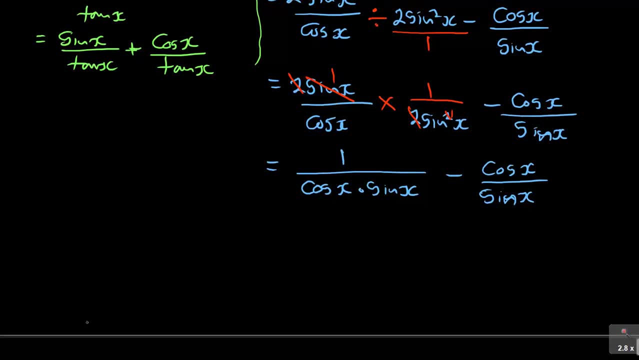 this part is again the common denominator between the two. So if I focus on cos x, sin x and sin x, the common denominator in this is cos x. I'm just going to do there the common denominator, which is cos x times sin x. 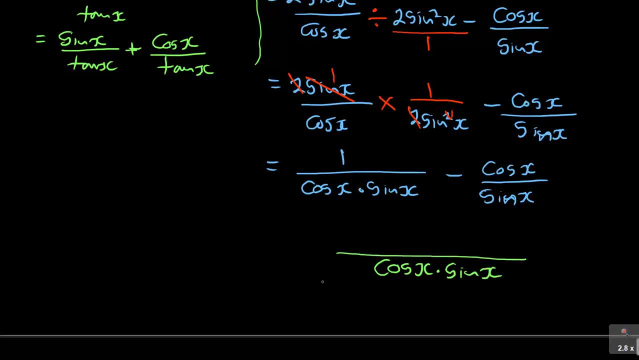 So that is the common denominator And you need to know fractions. So cos x, sin x into cos x, sin x is equal to 1.. 1 times 1 minus sin x into cos x, sin x will be the sin x will cancel the sin x. 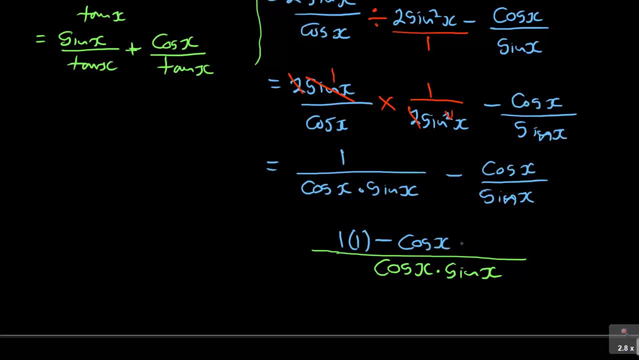 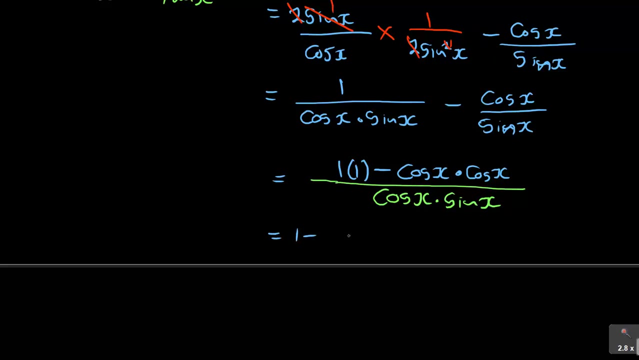 so that there is cos x remaining And then times the numerator, which is cos x, So that is what is still remaining on top. So when I simplify that 1 times 1 is equal to 1 minus cos squared x all over. 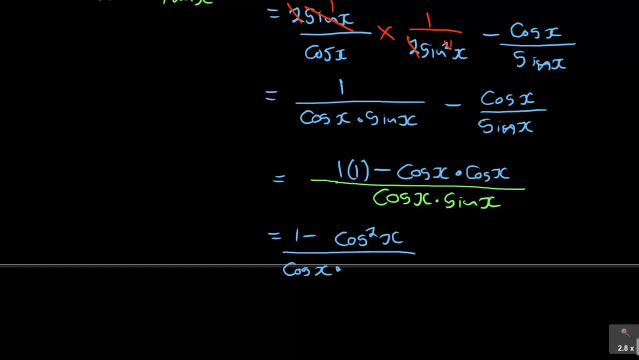 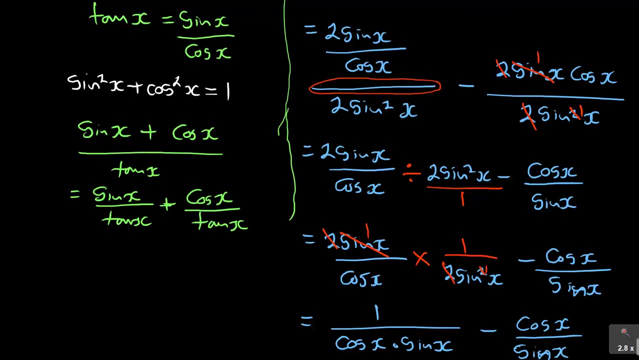 and then I've got cos x, dot sin x. And then this continues to say: now I've got 1 minus cos squared x. And, as I said previously, you need to know such identities. Now look at this identity, which is sin squared x. 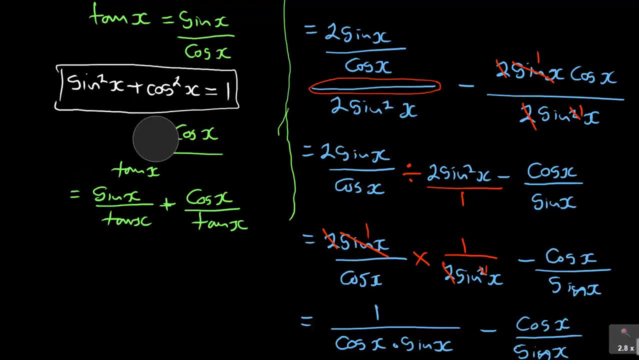 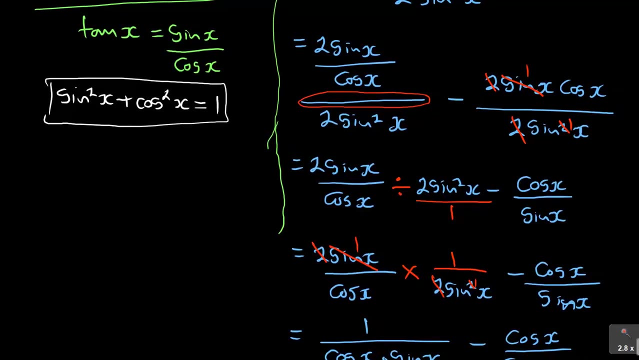 plus cos squared x, And if I can write it in by taking, for example, the sin squared. let me just check here by taking: yes, if I can take the cos squared instead to the other side of the equal sign. 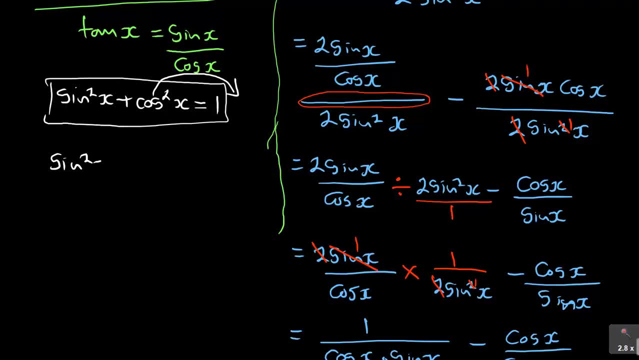 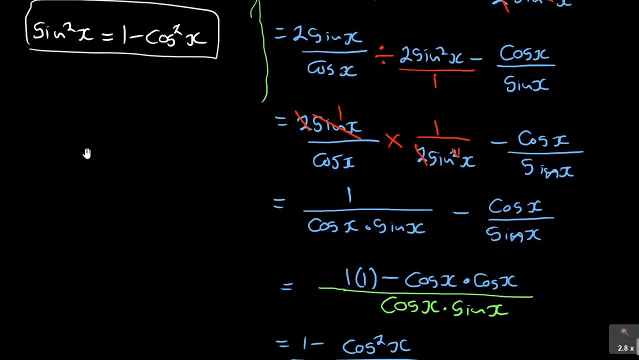 I will have: sin squared x is equal to 1 minus cos squared x. So now, if you look at this, it is what I am now having here at the bottom. If you can just check, this is what I'm having here, which is now 1 minus cos squared. 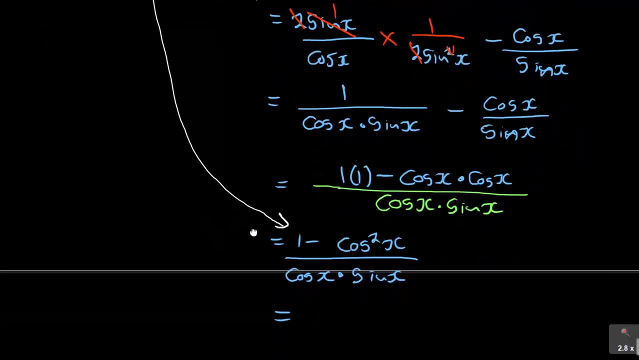 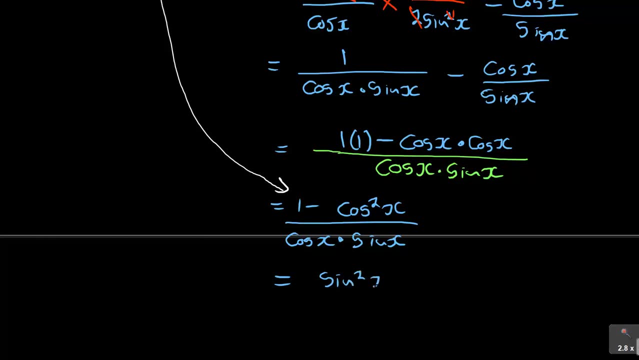 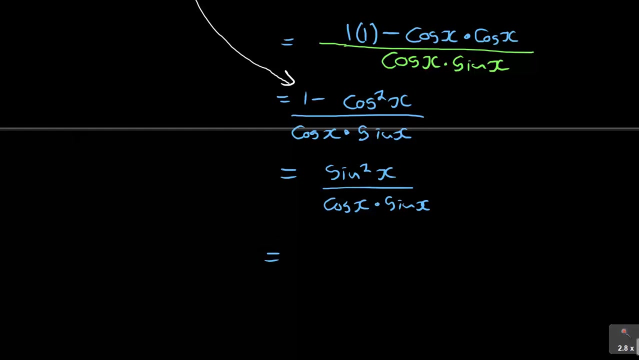 So this is equivalent or equal to sin squared x. So I can then continue to say: this is sin squared x over cos x times sin x, which continues to become equal to now. you can again cancel. the sin x will cancel.